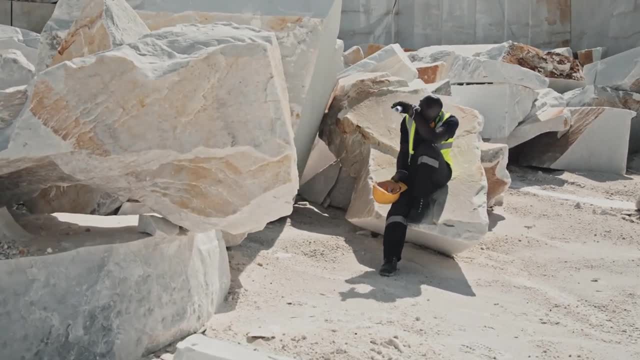 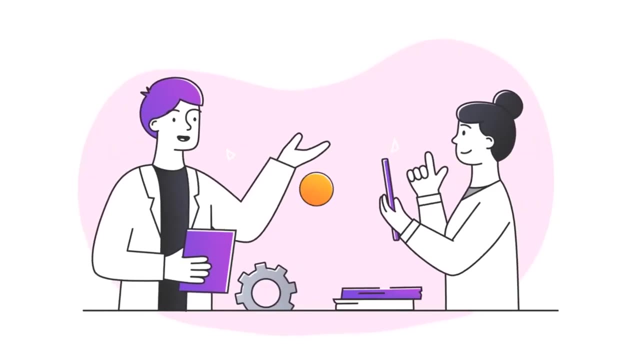 Hi, I am Tanning Emanuel, your online geology teacher from GBHS Mara, North Cameroon of Central Africa. In this channel, we share share videos based on scientific research and innovations, so make sure you subscribe to it if you truly need well-refined knowledge in science. 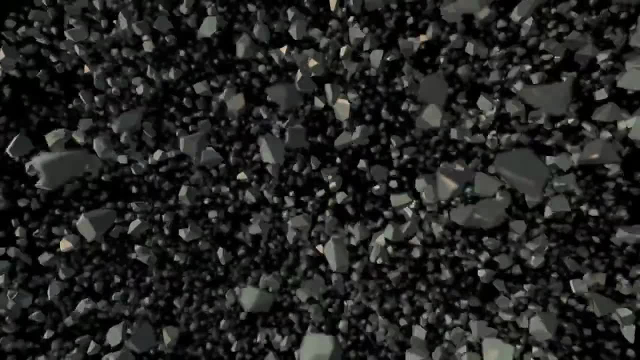 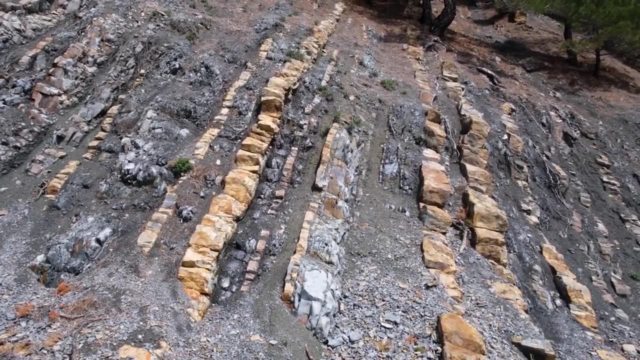 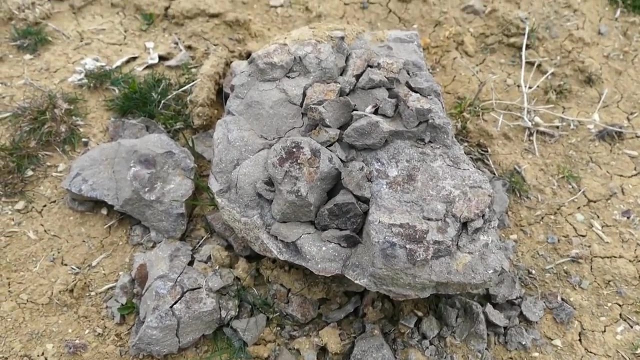 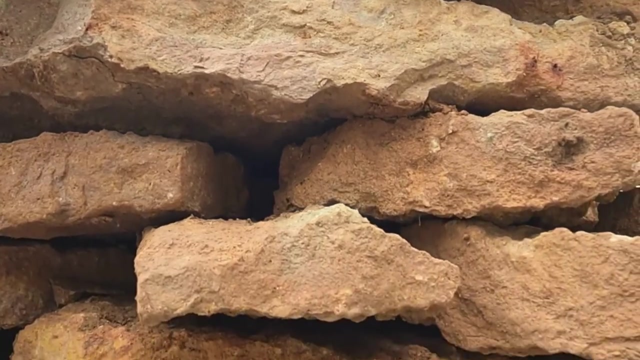 In this video, I will be focusing on how rocks response to stress. Rocks respond to stress through a process known as deformation. Deformation occurs when rocks undergo changes in shape or volume in response to applied forces. There are three main types of deformation that rocks can experience: elastic deformation, ductile deformation and brittle deformation. 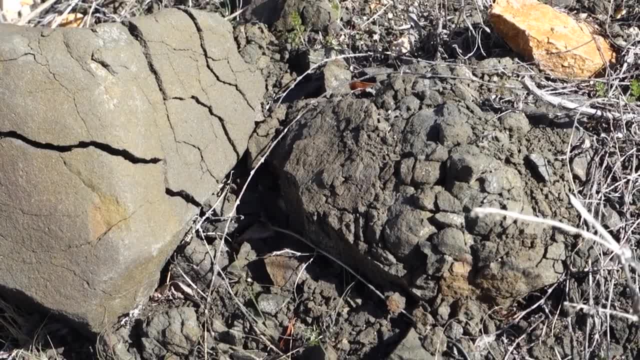 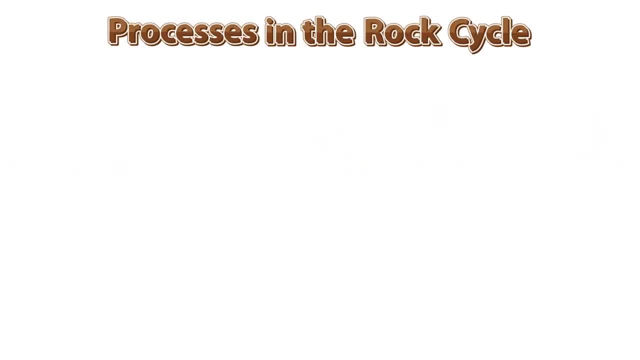 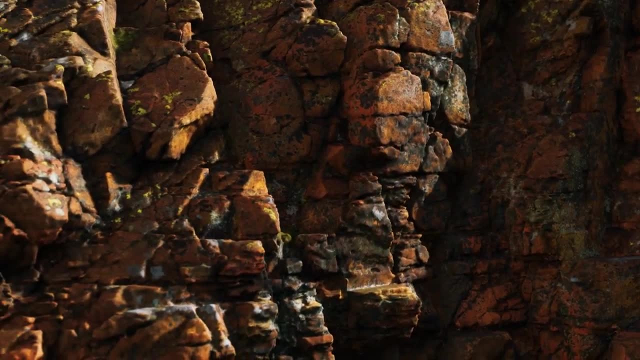 Elastic deformation. when a rock is subjected to stress, it initially deforms elastically. This means that the rock changes shape under stress, but can return to its original shape once the stress is removed. The atomic structure of the rock allows it to temporarily stretch or compress without permanently altering its shape. 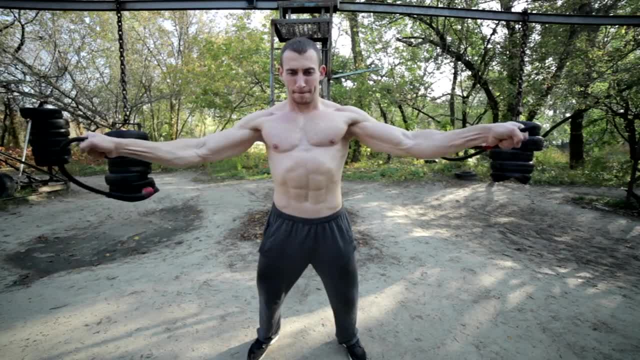 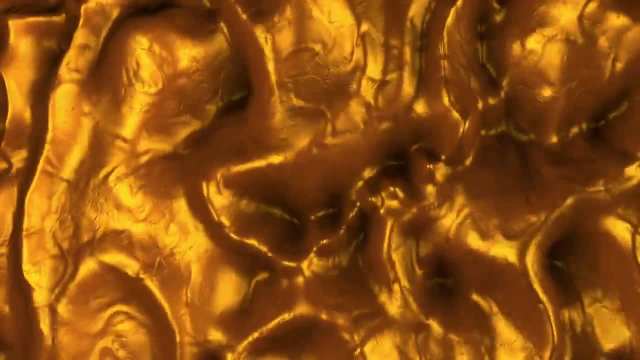 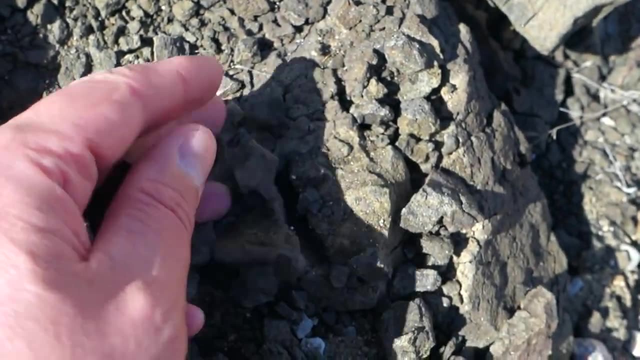 This behavior is similar to stretching a rubber band and then releasing it. Elastic deformation is reversible and does not involve the permanent rearrangement of mineral grains. Ductile deformation: if the applied stress is sufficiently high and the rock is subjected to prolonged periods of stress, it can undergo ductile deformation. 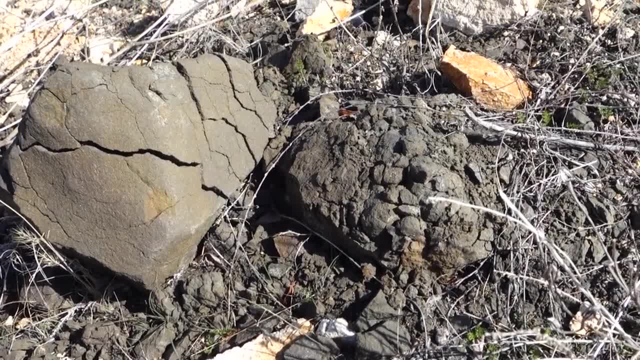 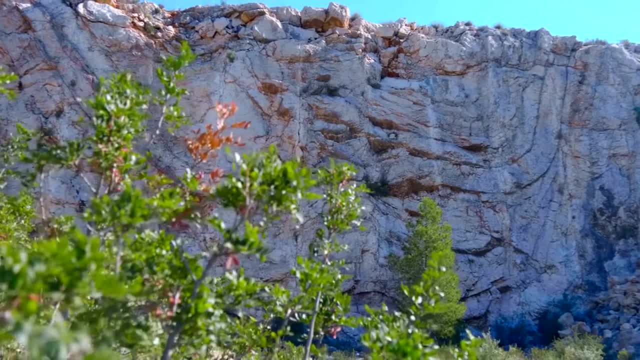 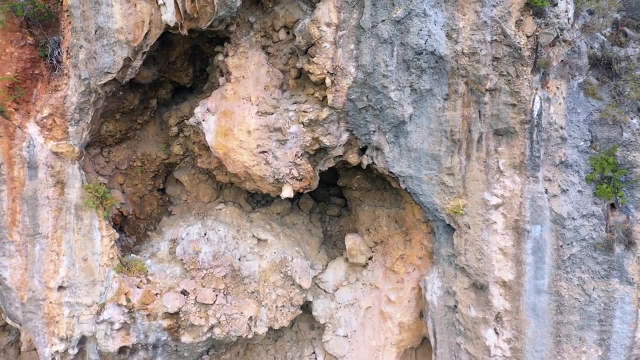 Ductile deformation occurs when rocks change shape by flowing or bending rather than breaking. This type of deformation is commonly observed in rocks that are found deep within the Earth's crust. where temperatures and pressures are high, The mineral grains in the rock can undergo permanent rearrangement, resulting in the development of new structures such as folds and foliation. 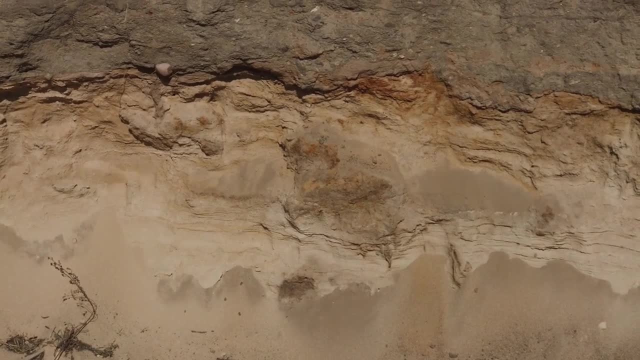 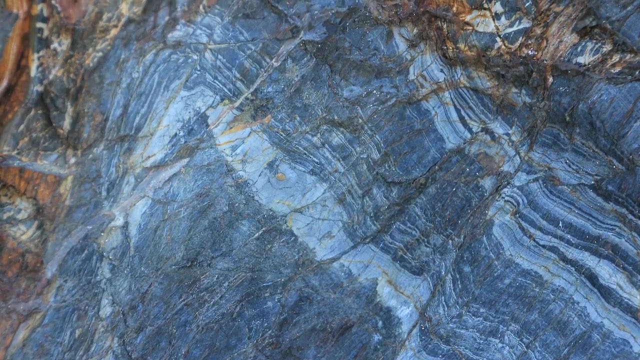 Brittle deformation. when rocks are subjected to high stress but over-arrangement In a relatively short period, they can undergo brittle deformation. Brittle deformation involves the fracturing and breaking of rocks along planes of weakness such as faults or joints.